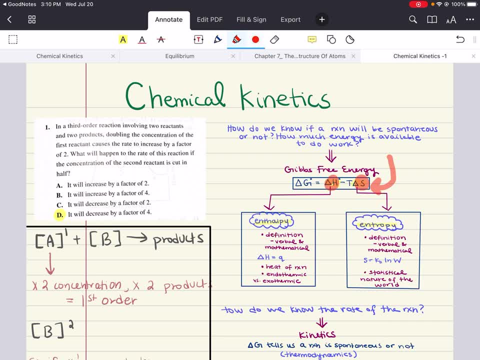 to give us a lot of information about the thermodynamics, The thermodynamics of the system, and whether our reaction will be spontaneous or not, whether it will occur or not, all right. So this change in Gibbs free energy is going to determine whether or not a reaction is spontaneous. all right, 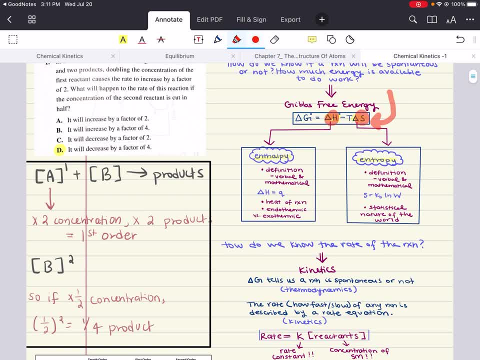 Now enthalpy, definition-wise, all right. heat of a reaction- delta H, that's enthalpy- is equal to heat, And we talk about endothermic versus exothermic when we discuss enthalpy. So does the reaction absorb heat or does it release heat? all right, And that determines. 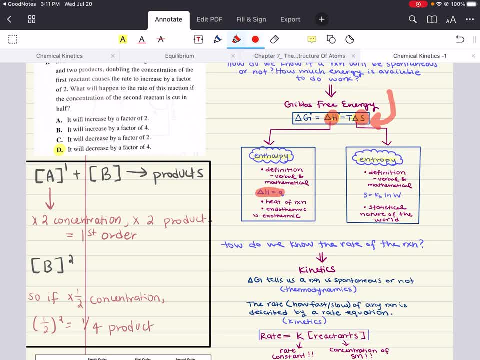 our value of delta H, whether it's positive or negative, And that ultimately has a role in what our delta G is, because if it's negative, then it's spontaneous, But if it's positive, all right, it's not spontaneous. Entropy is a little bit more of a difficult topic. 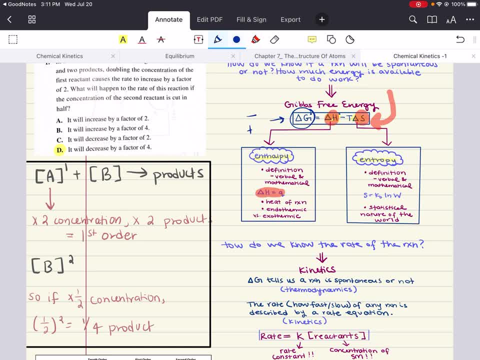 Most of the time you hear it's like the measure of disorderness in a system. all right. It's more so of stability, It's more of a statistical nature. whether it's more of has a statistical definition, all right. But in essence there are factors that help you determine whether the entropy. 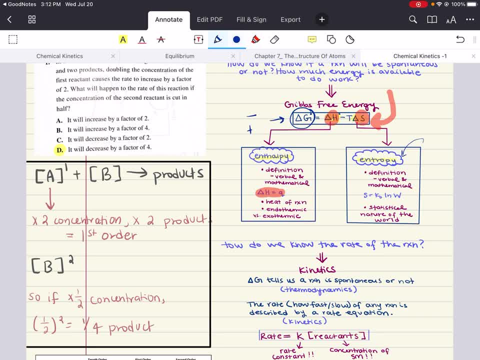 of a reaction increases or not. One thing is: if you create more product than reactants in terms of mole, that results in a positive entropy And, again, ultimately has a role to play in what your Gibbs free energy is, which ultimately determines whether or not. 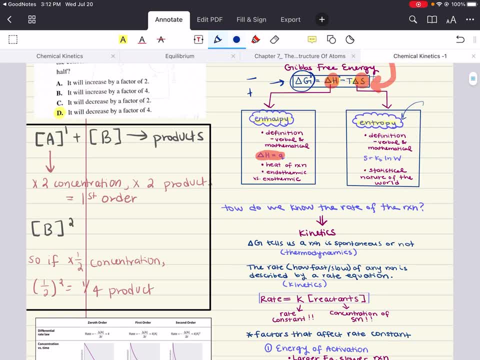 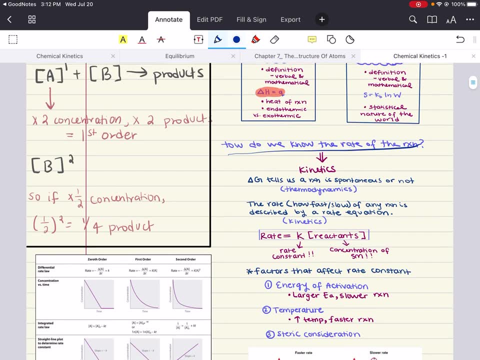 a reaction is spontaneous, Wonderful. So we can figure out what the entropy of a reaction is. So we can figure out what the entropy of a reaction is. So we can figure out whether a reaction is spontaneous or not. But how do we know the rate of the reaction? right, This is where chemical kinetics pops. 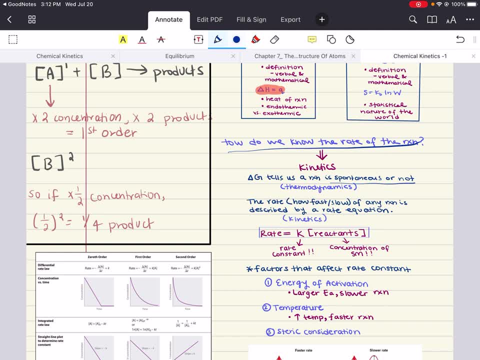 in right. Delta G tells us the reaction is spontaneous or not. That's the thermodynamics Cool, The rate, how fast or slow any reaction is, is described by a rate equation. All right, And this is our kinetics discussion here. All right, Now. the rate of equation is usually: 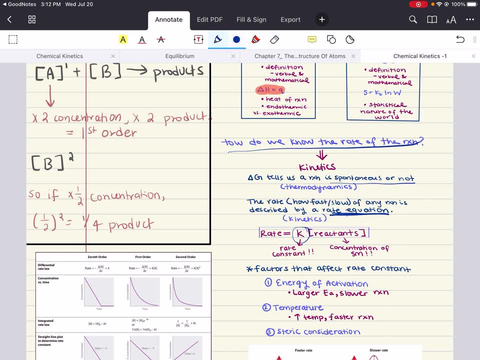 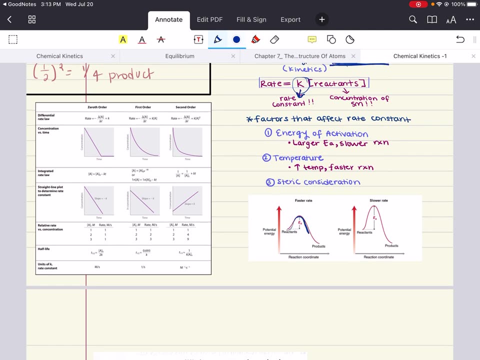 your rate constant multiplied by your concentration of starting material or reactants And the factors that affect your rate constant. for example: all right, is the energy of activation. All right, How much energy is required to activate the reaction? All right If this energy of activation is high. 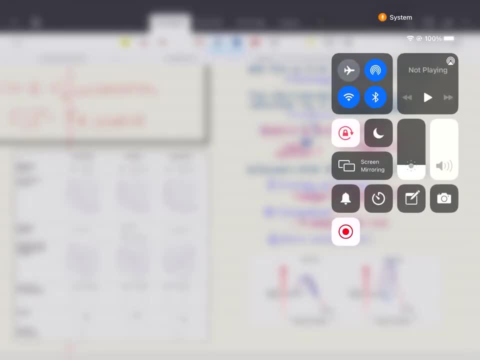 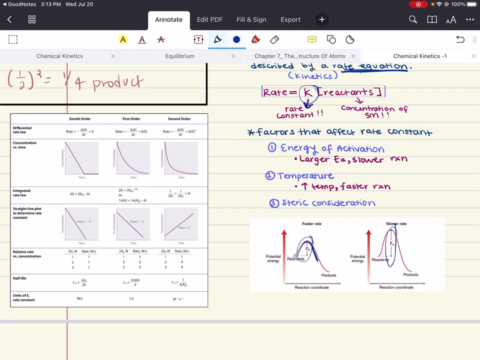 all right, the reaction is going to happen at a slower rate. Let me turn up the brightness for this. If the activation energy is low, then the reaction usually tends to happen at a faster rate. Temperature has an effect. If you increase the temperature, all right, the faster the reaction. 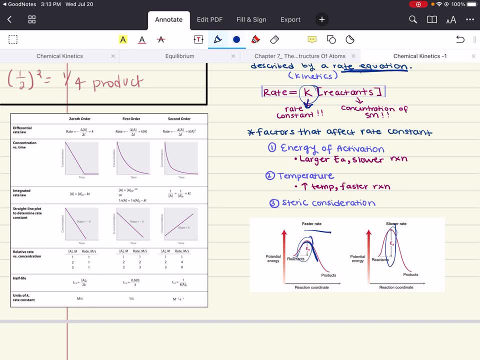 All right. Other things that affect the rate of your reaction are catalysts, things that you introduce that won't interact with the reaction itself or alter it in any way, but it will increase the speed by lowering the activation energy. All right, So conceptual. 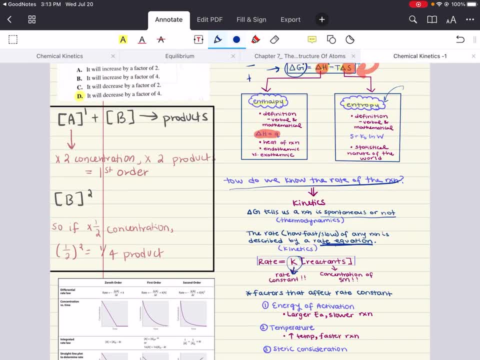 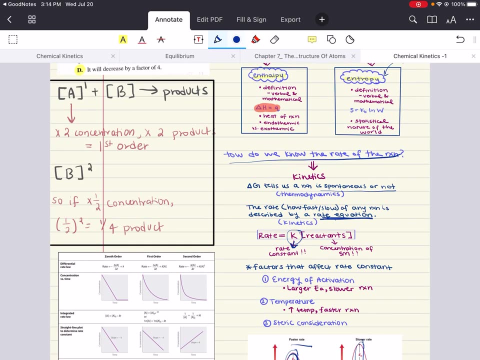 how you think about reactions, all right. There's a thermodynamic aspect, whether it's spontaneous or not, and there's a kinetics aspect: If it is going to happen, how fast or how slow is it going to be? all right. So that's important. Now, reaction rates, all right, or rate equations. 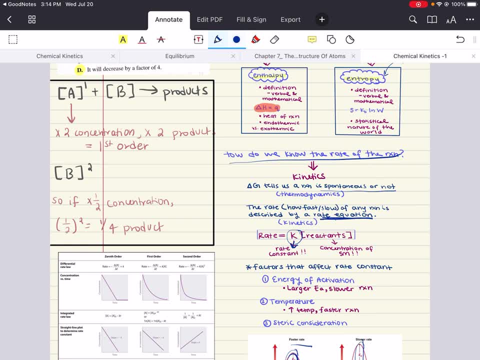 these are important. Reaction rates are measured in terms of the rate of disappearance of a reactant or appearance of a product. And rate laws take the form right, take the form that we see here. that rate equals a rate constant times the concentration of your starting material. 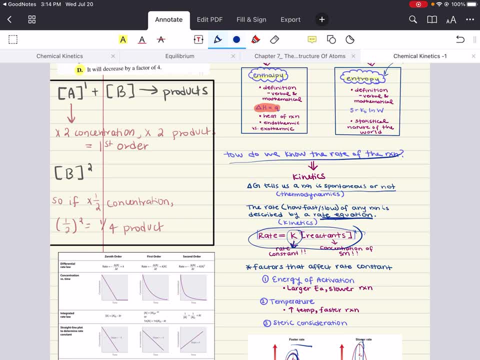 all right, And sometimes there's exponents associated with that, so that you can get the rate order of the reaction all right. The rate orders are important so you can tell whether your reaction is a zero-order reaction, first-order reaction, second-order reaction or third-order reaction, And those are important to be able to distinguish. 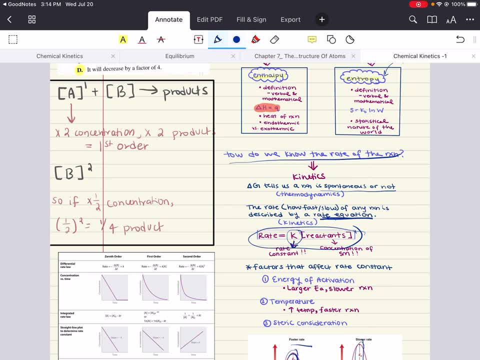 because whether you have a zero-order reaction first, second or third is going to play a role. if you increase one reactant, what happens to the product? If you increase both reactants by a factor of two, three, four? whatever, what happens to the product? Do they also vary linearly? 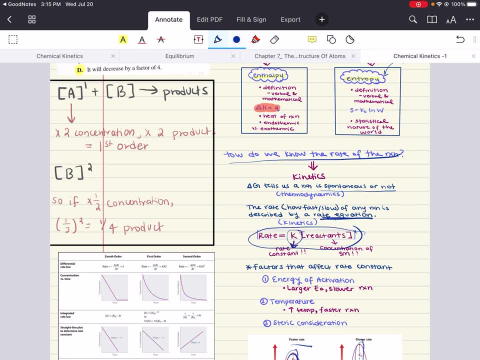 exponentially. What's the ratio? Well, that depends. It depends on what kind of order reaction you have And hopefully, through covering these problems, we're going to be able to talk about each one of these order reactions, especially zero one. 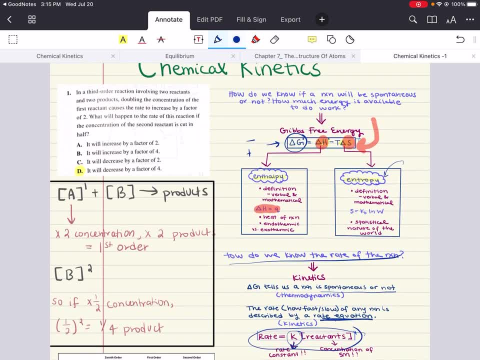 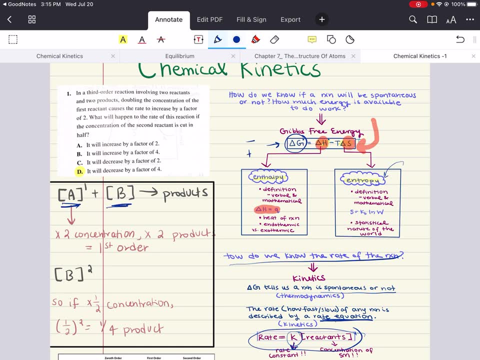 and two. all right, These are your most important ones. okay, Now, with that background information, let's look at this problem again. Third-order reaction: you have two reactants, all right, and you have two products, whatever Doubling the concentration of the first reactant. let's call it. 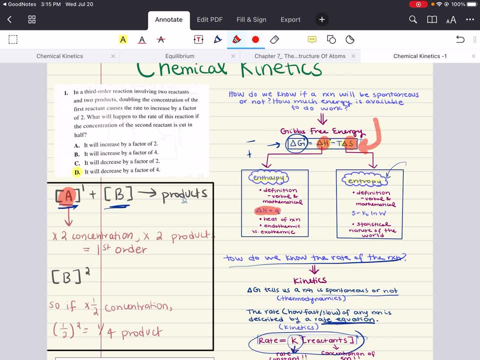 A all right First reactant. You double the concentration, cool. So you multiply it by two. all right, And guess what? You also double the rate. okay. So if you double the concentration of the first reactant, it causes the rate to increase by a factor of two. all right, So times two in terms of rate. 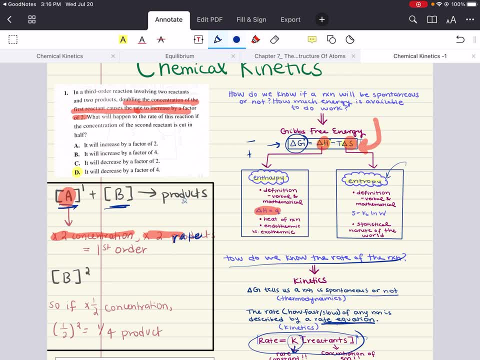 all right, Cool, When you increase this, when the rate is um, when the concentration of the reactant, the reaction doubles and then the rate also doubles. what kind of order are we talking about? when things factor and scale up proportionally, You increase concentration by two, you increase. 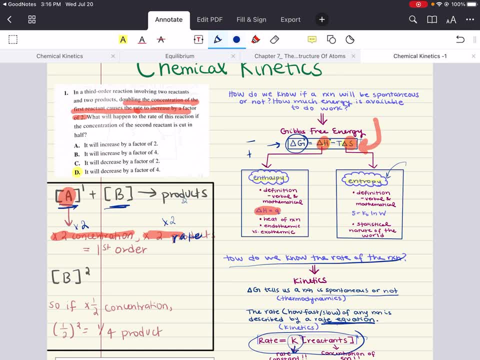 the rate by two. This is the description of the rate, that the rate is first order with respect to the concentration of the first reactant. okay, Because doubling this reactant also doubled the rate. all right, They scaled exactly the same. Then the rate is first order with. 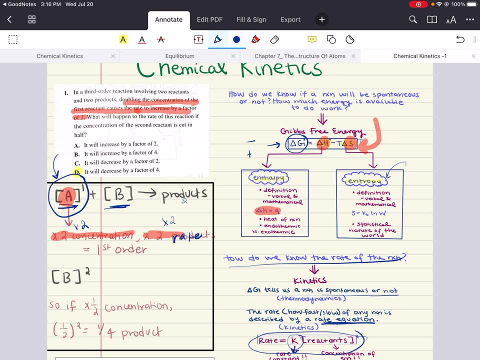 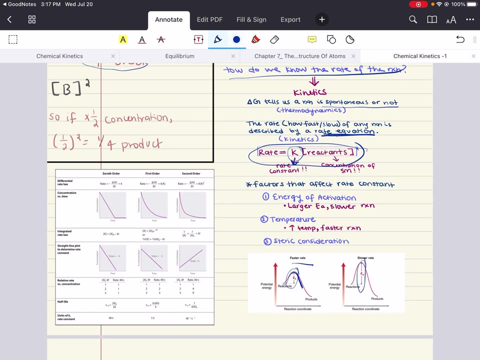 respect to the concentration of the first reactant, all right. So the first reactant, all right, is working in the sense that it is the first order, all right, And if you remember first order reactions, all right. have a non-constant. 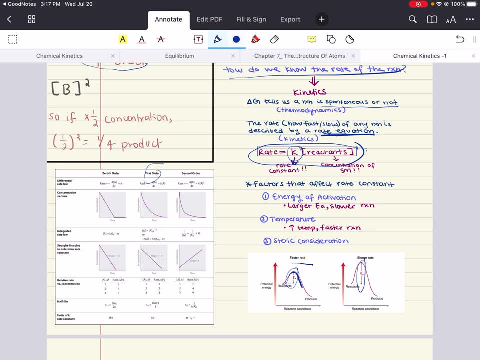 rate that depends on the concentration of reactant, all right. So what you notice is the concentration versus time curve of the first order reaction is non-linear, all right, And the slope of the log concentration versus time plot is minus K for the first order reaction. 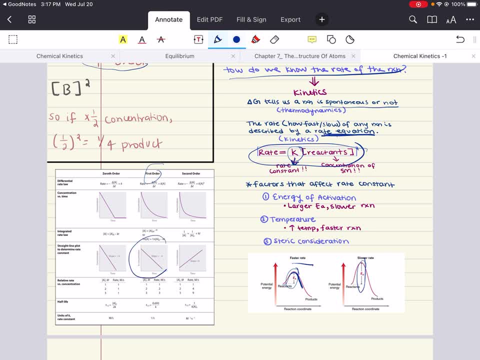 all right. So if you look at, all right, the log versus time or log versus, yeah, the log versus time plot for the first order, all right. we have minus K for first order, all right. It has a non-constant rate that depends on the concentration of reactant, all right. And if we have a, 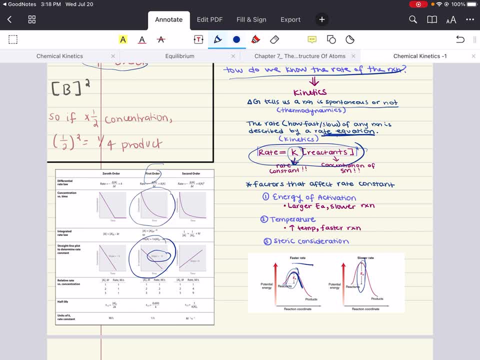 concentration versus time plot. what you notice: it's non-linear. all right. Something else that you should notice is, all right, relative rate versus concentration. all right, It scales. all right, You double the concentration, you double the rate. 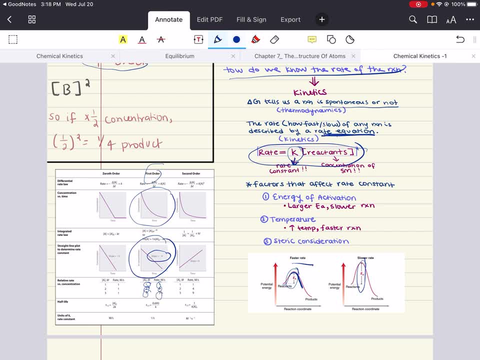 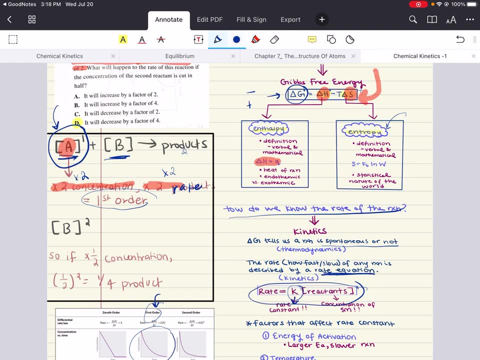 all right, You triple the concentration, you triple the rate. all right. That's an important thing that you need to remember about first order: all right. That's why we can say, based on the information given, the rate is first order with respect to the concentration of the first. 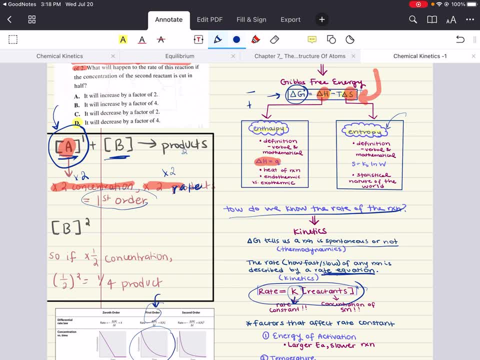 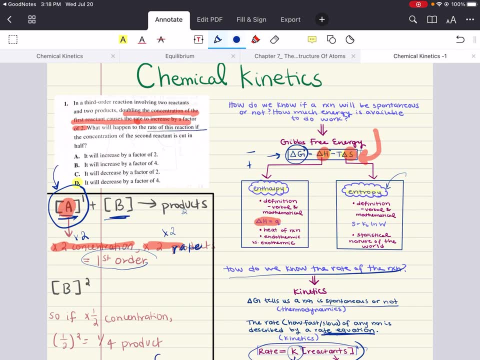 reactant. If the concentration of that reactant doubles, guess what? The rate also doubles, Cool. Well, what will happen to the rate of reaction if the concentration of the second reactant is cut in half? Okay, this is great. We figured out one reactant. all right, is first order, all right. 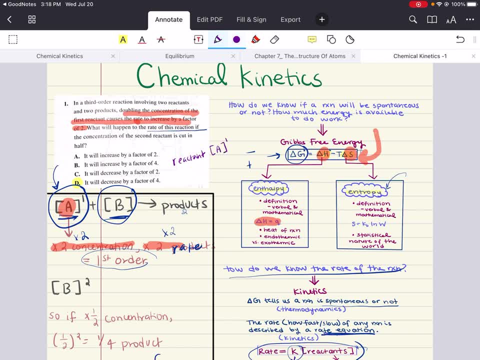 That means it has a one coefficient here. all right, for A whatever it might be all right. But we have another reactant. all right, We don't know what the coefficient to the second reactant is, but guess what? We don't know what the coefficient to the second reactant is, but guess. 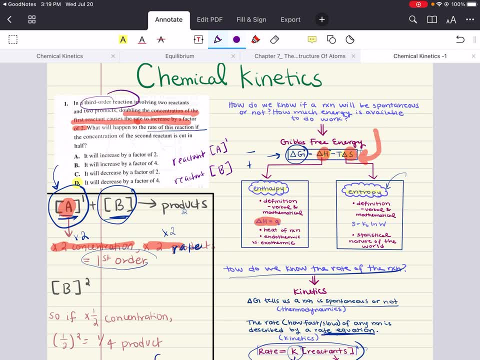 what We know, the total order of the reaction. The total order of the reaction is third order. That means the coefficient for reactant 1A and reactant B has to add up to three. So that means the second reactant is a second order. a second order, all right. with respect to the concentration. 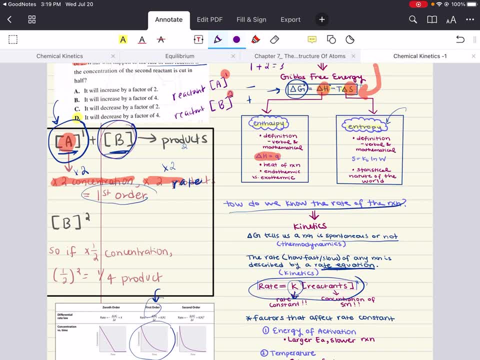 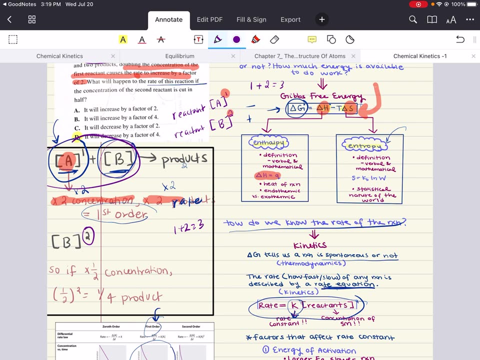 of the second reactant, all right. So the second reactant is second order, all right. One plus two equals three. The whole reaction is third order. Perfect, all right. Perfect. Remember, we can tell what order our reaction is based off of summing, all right. summing the coefficients. 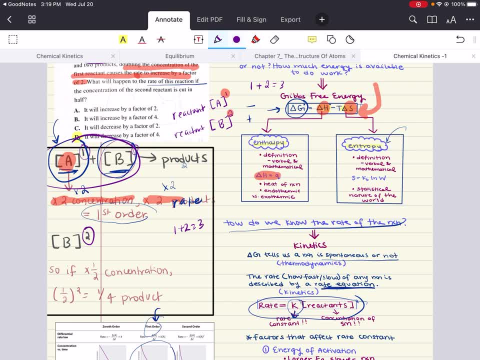 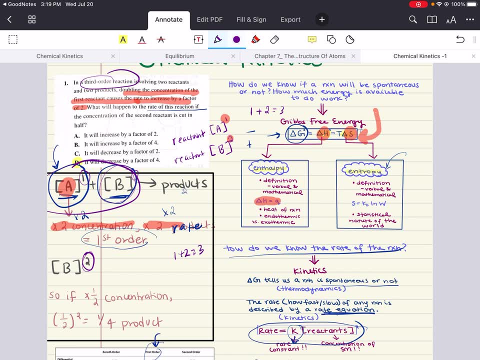 of our reactants. all right, Perfect. So then, if B is second order, how do things scale in terms of when you change the concentration? how does the rate? how is the rate altered? Well, we know that the concentration of the second reactant it's cut in half. 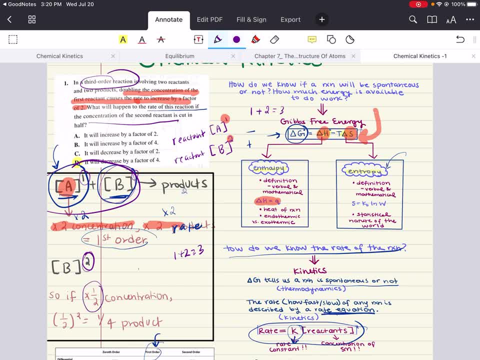 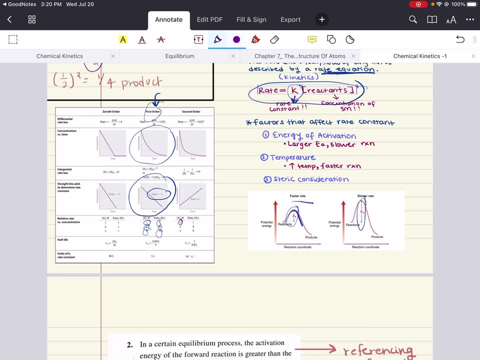 all right. So what we're taking is we're multiplying the concentration by one half, because we're cutting it in half. all right. In second order reactions, what happens is things scale exponentially. all right. So if you have a concentration, if you multiply your concentration, 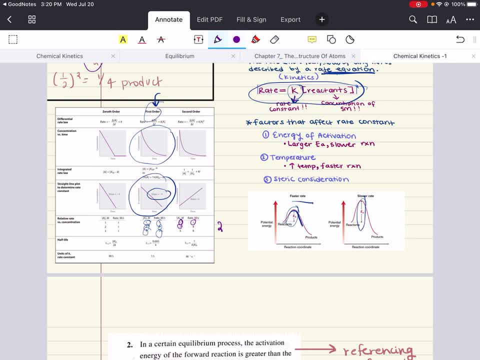 by two. all right, the rate is squared, All right. so if you change the concentration by two, the rate changes by an order of four. If you triple the concentration, the rate changes squared. So the rate of reaction is changed by a. 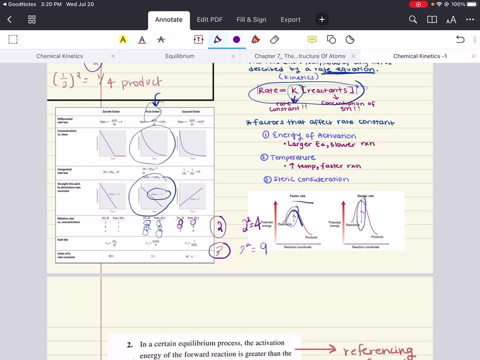 factor of nine, three squared, all right, And so on and so forth. all right, So it scales exponentially squared, exactly all right. So if we cut the concentration of reactant B by one half, guess what happens If we cut the concentration of reactant B by one half? 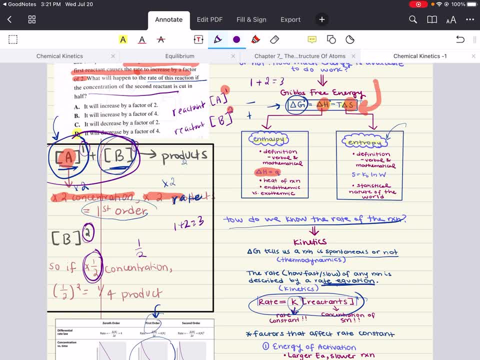 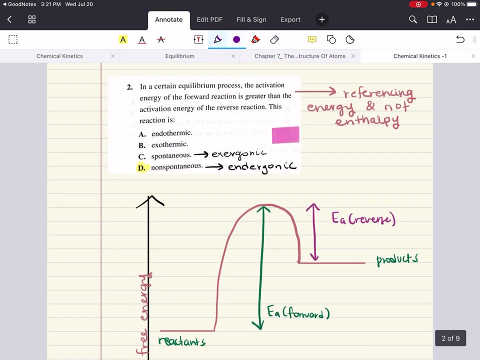 how much the rate of the reaction has changed. One half squared one fourth. We cut the rate by one fourth, It will decrease by a factor of four. All right, So the correct answer is D. All right, Fantastic. Let's look at question two. In certain equilibrium process, 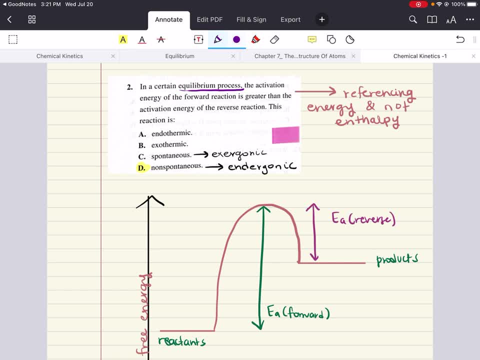 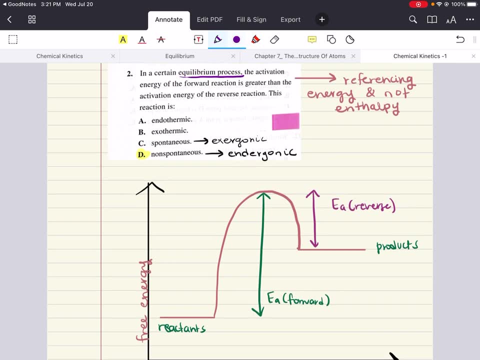 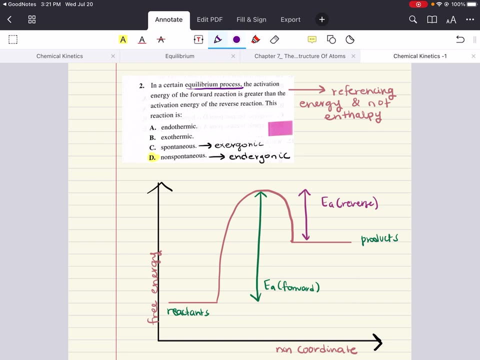 the activation energy of the forward reaction is greater than the activation energy of the reverse reaction. All right, This reaction is blank. All right, Fantastic. So this is in a certain equilibrium process. the activation energy- All right, It's referring to energy and 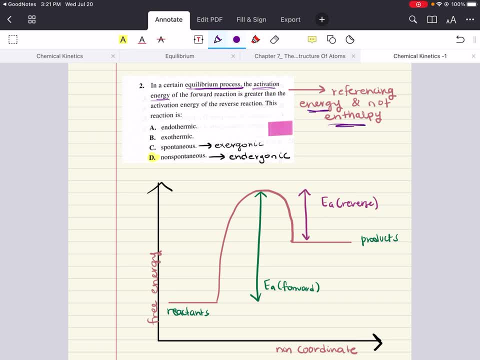 not enthalpy. All right, This is a very important first thing that your eyes have to catch. It is discussing energy, not heat or enthalpy. Okay, This is going to help you cross out two answers off the bat, All right, And these two: 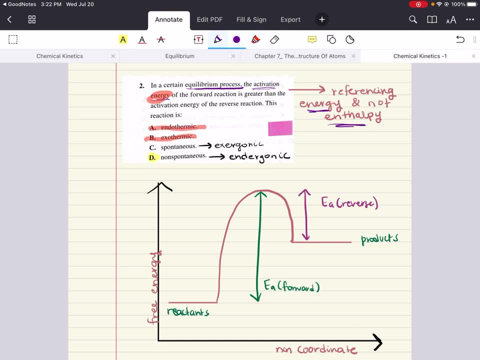 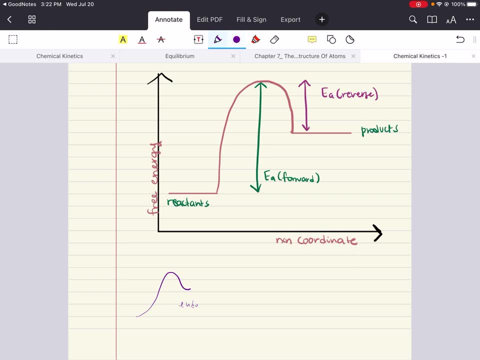 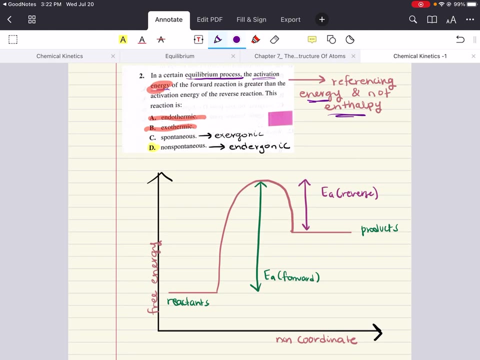 answers are endothermic and exothermic. You cross that out. Why You're not talking about a heat diagram and determining whether things are endothermic or exothermic. All right, You're not doing that. You are discussing energy here, The terms that you use when you're. 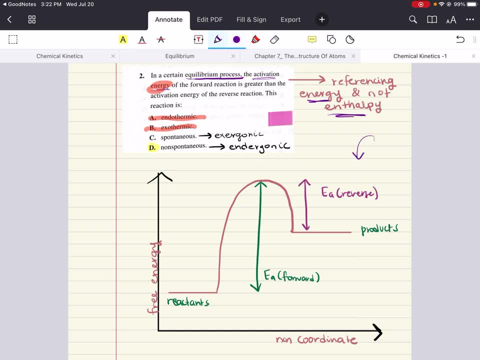 discussing an energy diagram are exergonic Or endergonic, And in other words, exergonic is spontaneous, where endergonic is also referred to as non-spontaneous. All right, These are interchangeable terms. All right. And when? 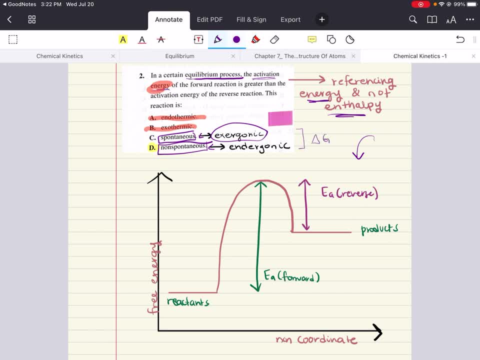 you're talking about energy here. you're talking about that, Gibbs, free energy. All right, So this problem, off the bat, gives you a huge hint that allows you to cross out half of the answers here. In certain equilibrium process, the activation energy of the forward reaction is greater than. 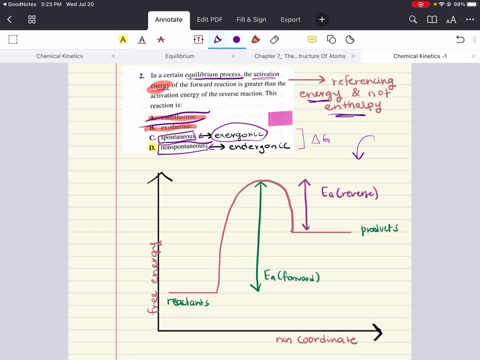 the activation energy of the reverse reaction. So this is a very important question. All right, We're talking about energy, And when you describe energy diagrams, you are either using endergonic versus exergonic or, similarly, spontaneous versus non-spontaneous. All right, 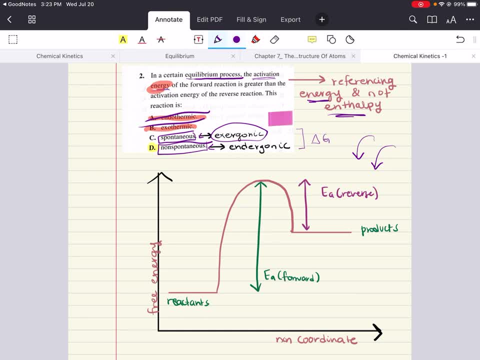 So important thing to note off the bat. All right, Cool, Now I drew what this diagram looks like. Okay, It says the activation energy of the forward reaction is greater. All right, Then the reverse. So if you're You're starting off as reactants here from the start, All right, And you're going to end. 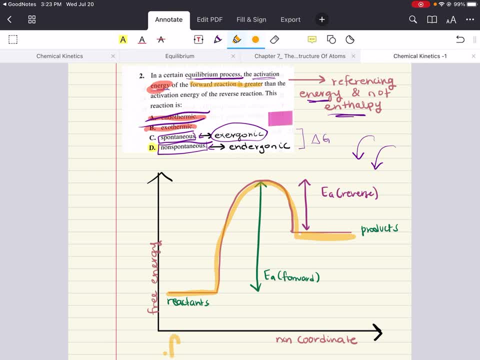 products. All right, The forward reaction is drawn here in orange. Okay, That forward reaction should have a greater activation energy than the backward reaction. I'm going to draw you the backward reaction now. All right, The backward reaction is pretending your products are actually reactants. 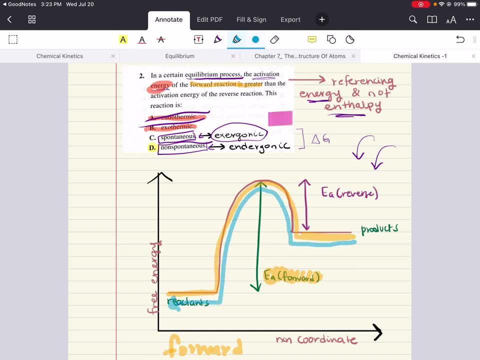 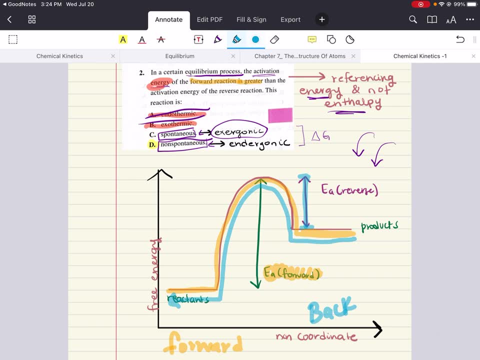 now and going backwards. All right, Look at the activation energy for the backward reaction. That's it. That's the activation energy, The barrier of energy that it has to surpass to complete the reaction. And look how we drew this appropriately: where the forward reaction. 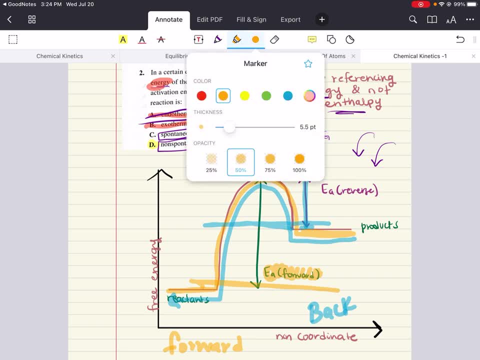 clearly has- All right, Clearly has a higher activation energy than the backwards reaction. Cool, So we were able to draw it with the hints that we were given. Now we have to be able to describe it using the terminology: All right. Now, if the activation energy of the forward reaction is greater than the activation 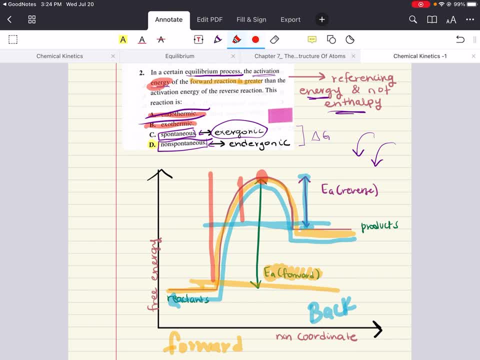 energy of the reverse reaction, then the products must have a higher energy than the reactants. That's something you should keep in mind in case drawing this was hard. All right If the activation energy of the forward reaction is greater than the activation energy of the reverse. 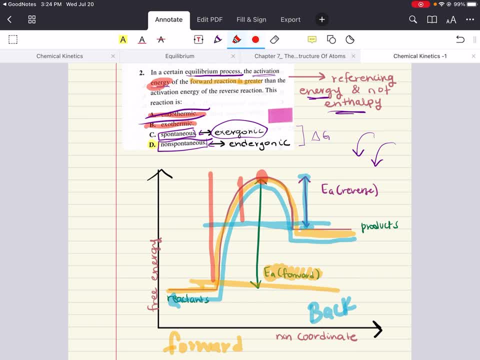 reaction, then the products must have a higher free energy than the reactants. Overall energy of the system is higher at the end than it was in the beginning. All right, Now the net free. energy change is positive. All right, The net free. I'm sorry. 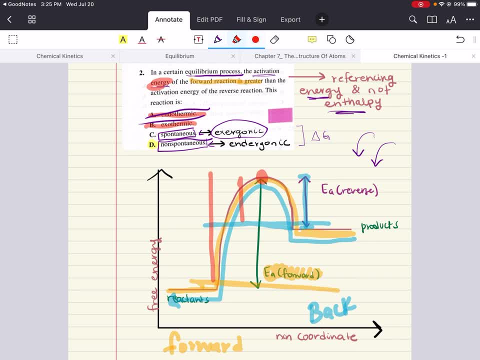 The net free energy change is positive. All right. You're ending up with higher than you started off in the reactants, All right. So this is delta G positive. Sorry, I should write that better. All right. Positive Final minus initial where final is greater than initial. 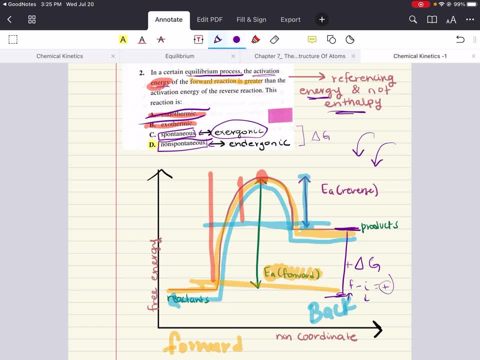 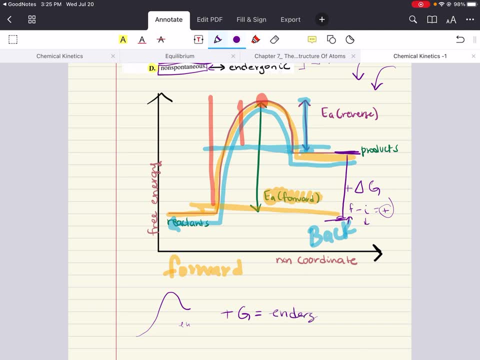 is going to give you a positive number. You're going to have a positive Gibbs free energy, All right. And a positive G is an endergonic process. A negative delta G- Sorry, I didn't draw the deltas. This is an exergonic reaction. It's kind of similar to enthalpy. If you have a 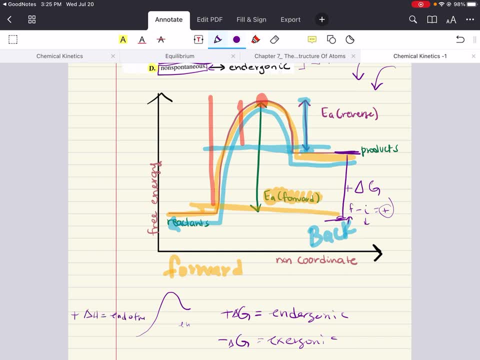 positive delta H, it's endothermic reaction. If you have a negative delta H- enthalpy, then that's an exothermic reaction. And that makes sense, Because if you gain energy, that means you absorbed it. It went in Endothermic, All right. 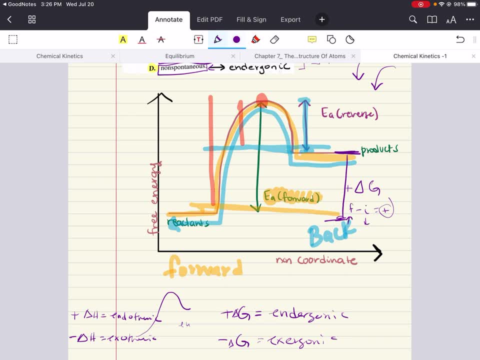 If you expel energy, all right, then that's exo, It's exiting, All right, And that's why you have a negative H, because you lost energy. Right Makes sense: Exothermic, Same thing You can. 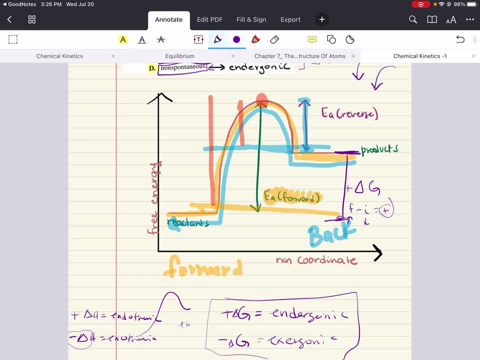 kind of use the same prefixes, to help you remember, with Gibbs free energy. If the Gibbs free energy is positive, it's endergonic, All right. And if it's negative, it's exergonic, like exit and enter. That's how it works, All right. And if it's negative, it's exergonic, All right. And if it's 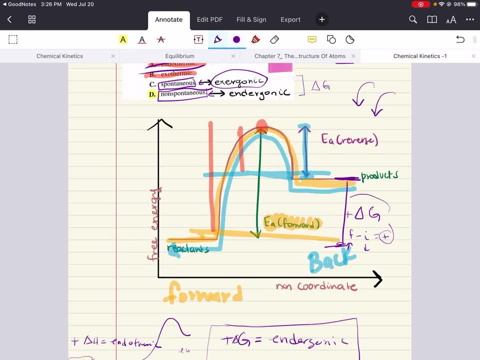 helps me remember it All right. So again we have a positive delta G here. right, Because your products are higher than your reactants. Final minus initial is going to be a positive value because your final is going to be like higher energy, like a thousand, For example. your lower. 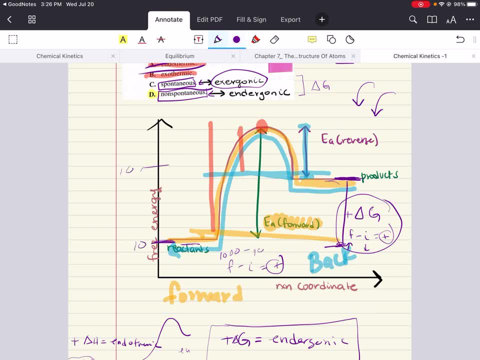 energy is going to be like a 10.. All right, I'm just throwing random numbers to help you visualize this mathematically, in case that's a problem. Right, That's going to always give you a positive number. Okay, So it's a positive. delta G. It's endergonic. What's the associated term for? 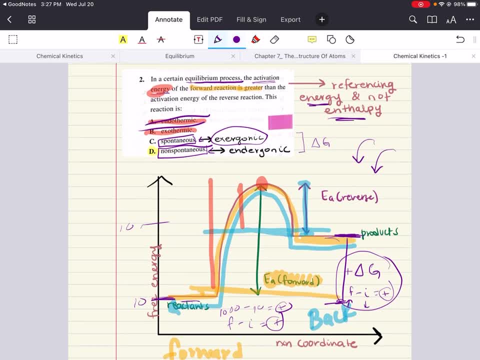 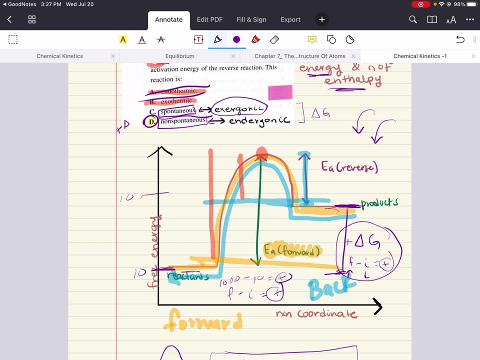 endergonic. Since endergonic is not an option choice here, All right. The synonym for that that's used interchangeably is non-spontaneous. Obviously right, Because you have a positive delta G. Positive delta G indicates non-spontaneous. minus delta G indicates spontaneous reaction. 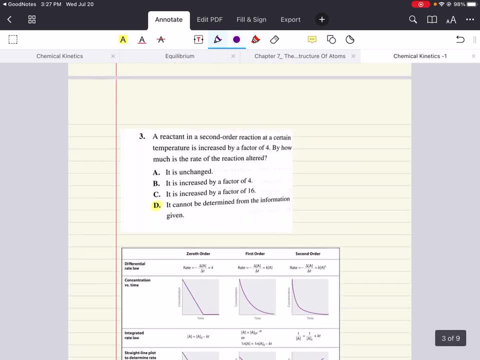 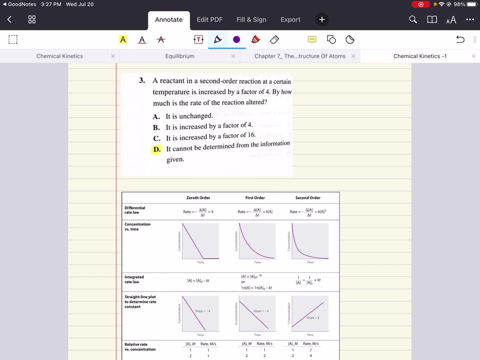 All right, Fantastic Answer is D. Now three says a reactant in a second order. reaction at a certain temperature is increased by factor of four. By how much is the rate of the reaction altered? All right, This is a tricky. 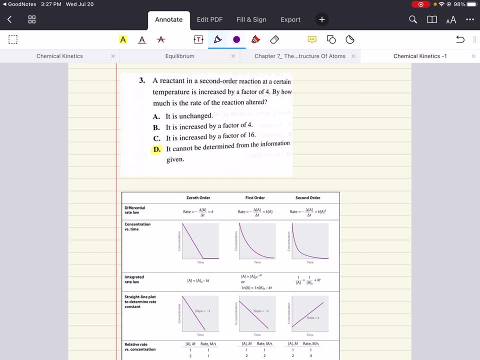 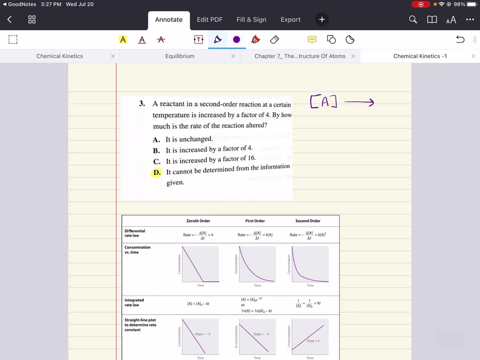 question. All right, Let's talk about this. A second order reaction can be second order with respect to one reactant or first order with respect to do different reactants. Let me put this in demonstration for you. All right, Let's pretend you have reactant A and it gives you. 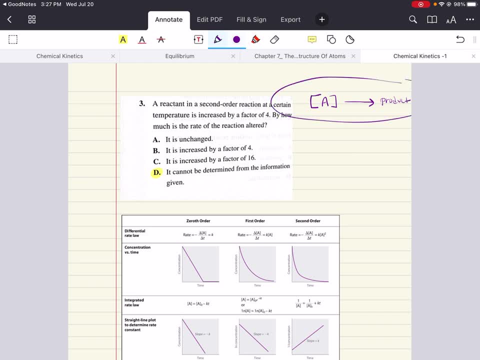 a product, All right. This kind of reaction can be second order. Actually, if the reactant A, the only reactant, the single reactant, is second order itself. Another way to have a second order reaction is to actually have two reactants. All right, That are. 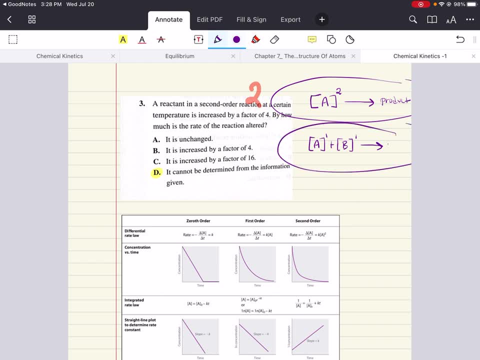 both first order each. Then the total order of the whole reaction is: one plus one equals two, All right. So there's two scenarios, at least right To have a second order reaction where you have one reactant that operates as if it's in second order, or two different reactants each. 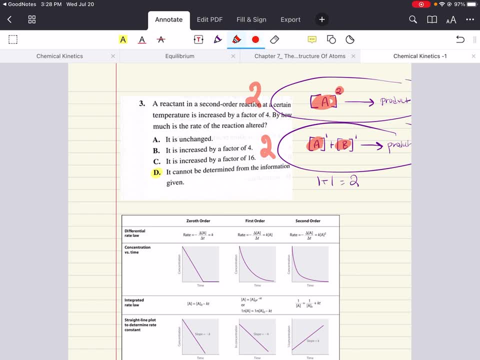 that are first order reactants and the total order of the reaction is second order. All right, So in this case, what they're saying, in this case one reactant was increased by a factor of four If the reaction- I'm sorry, it's saying a reactant in second order- reaction at a certain 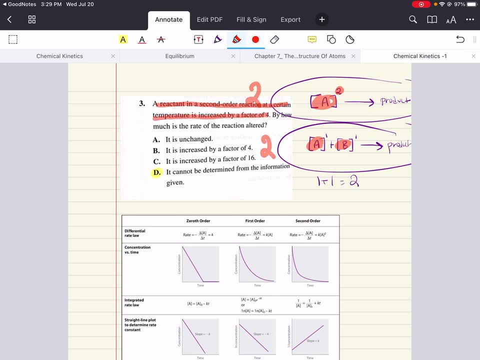 temperature is increased by by a factor of four, All right. So if one reactant was increased by a factor of four, if the reaction is second order with respect to the single reactant, all right, then the rate is going to increase by a factor of 16.. Remember, things in second order are gonna square All. 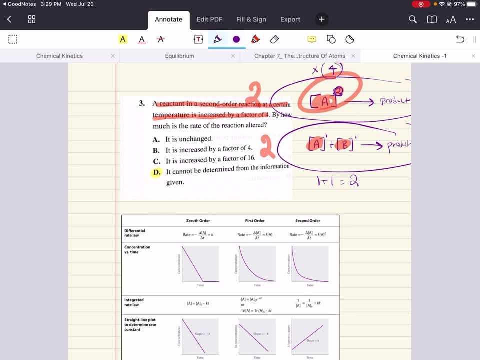 right, If you, if you change the concentration by four, the react, the rate of reaction, all right, uh uh. factors by square. So if you multiply the react, the, the concentration of a, which is a second order reactant, by four, guess how fast the reaction rate is going to increase. 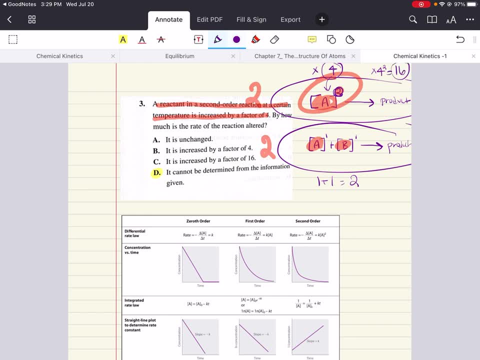 by four, squared by 16, orders by a factor of 16.. I'm sorry, All right, But if it is first order with respect to this reactant, all right, And first order with respect to another reactant, then the rate of the the rate is only going to increase by. 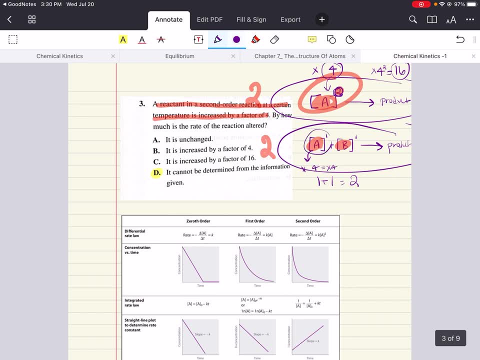 by four each. All right, Because remember first order. All right. If you multiply the concentration by four for first order, how does the rate factor by the same amount? All right. Now we don't know which case we're talking about. They don't tell us. 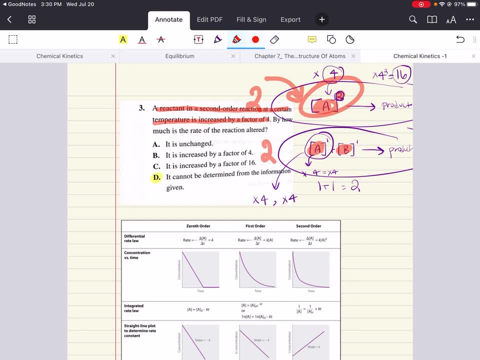 oh, we're talking about a second order react, uh reaction where there's only one reactant that is second order, or we're talking about a reaction that has two reactants each that are first order? We have no idea Which scenario they're talking about, So how can we possibly answer this question? 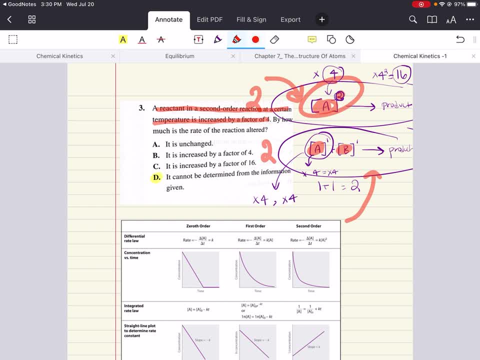 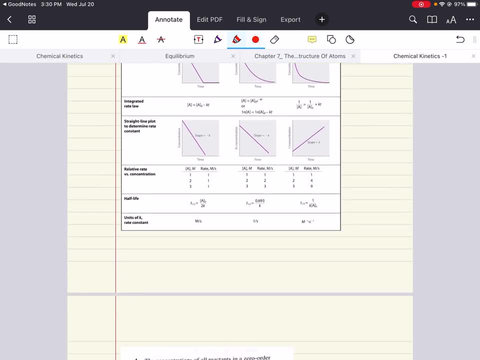 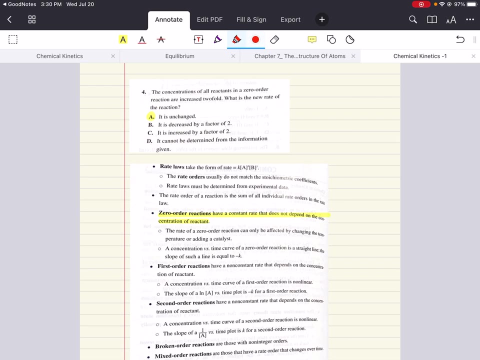 by how much is the rate of the reaction altered? There is not enough information to tell, And so the correct answer here is D. Fantastic. Let's move on to four forces. The concentration of all reactants in a zero order reaction are increased twofold. 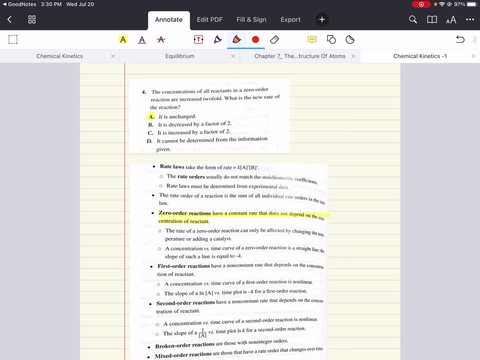 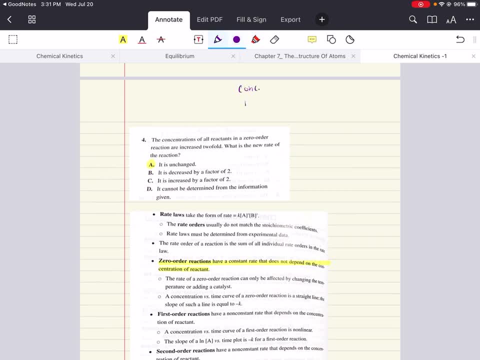 We've talked about what happens when you increase the concentration for first order and second order. What happens to the rate when that happens? All right, So if you increase the concentration of a first order reaction by an amount times- and it could be times to increase times three- 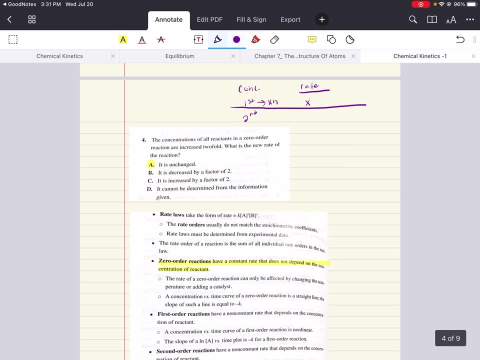 how does the rate work? for first order It also increases by the same amount. So in a first order reaction, if you double the concentration, you double the concentration, You double the rate of the reaction. If you triple the concentration, you triple the rate of reaction. Multiply by N. whatever times N, All right. 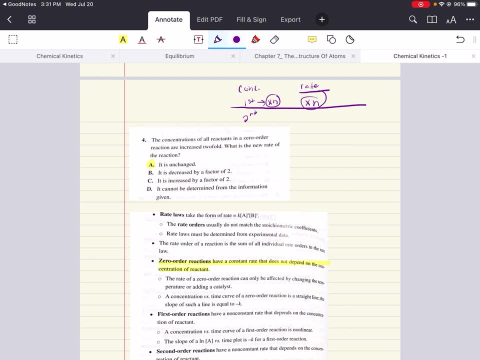 The concentration. you multiply by N for the rate With second order reactions, all right. if you multiply by times N, if you take a second order and you double the concentration, all right. how does it factor Squared? All right, So if you double the concentration of a second, 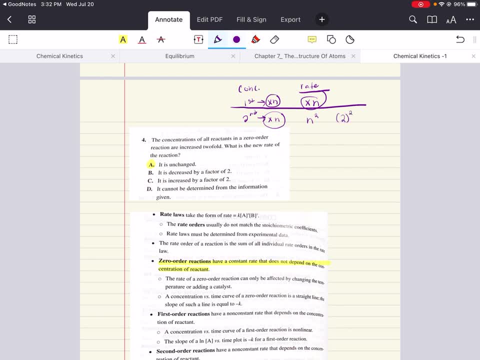 order reaction. then you square two, All right, And you increase the rate by four folds, All right. If you triple the reaction of a second order, all right. then the rate increases by three squared, or nine times is more In a second order reaction. if you multiply the concentration by 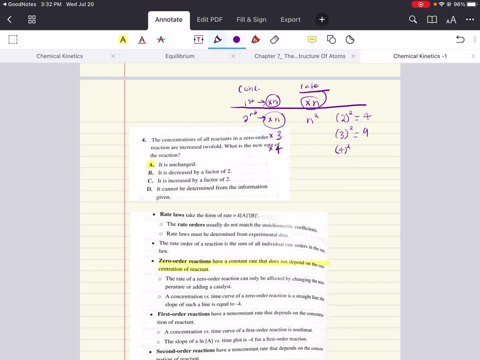 four, all right, then you four square the rate, That means you increase it by 16. Folds, Cool. But what about a zero order reaction? All right, This is my favorite order reaction. Whatever you do to the concentration has no effect on the rate. No effect on the rate whatsoever. So 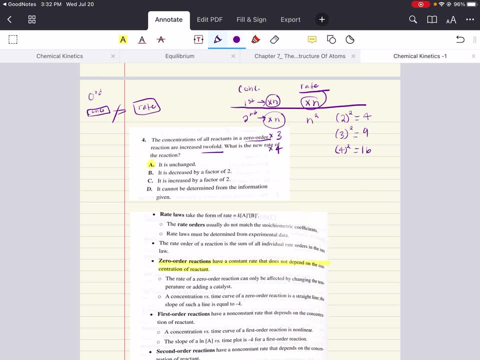 if we take a zero order reaction, we increase the concentration times two. What happens to the rate? Absolutely nothing, All right. Zero order reactions have a constant rate That does not depend on the concentration of a reactant, Thus changing the concentration of. 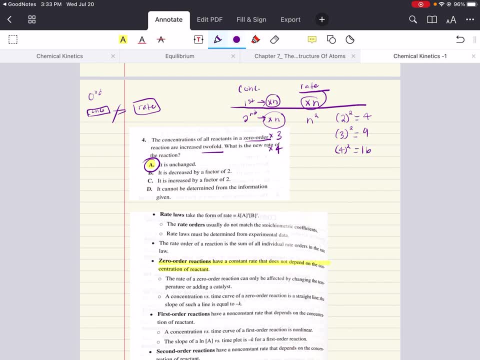 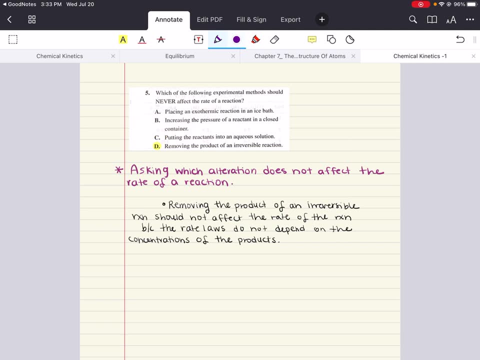 this reactant is not going to affect the rate. So the answer is A Fantastic. Let's do five now. Which of the following experimental methods should never affect the rate of a reaction? All right. So this question asks: which alteration does not? All right, We're going to ask, We're. 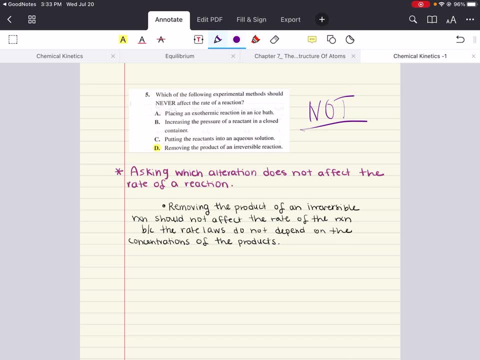 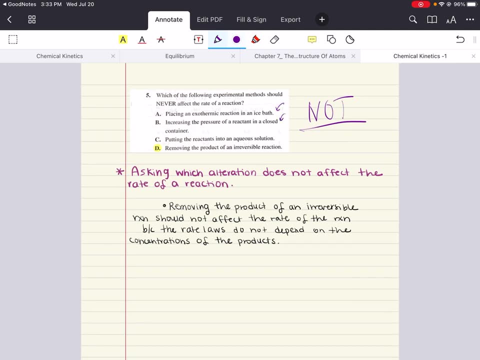 going to write, not in a big, In big capital letters Does not affect the rate of the reaction. Okay, What we're going to look at here. let's read the answer choices really quickly. A says: placing an exothermic reaction in an ice. 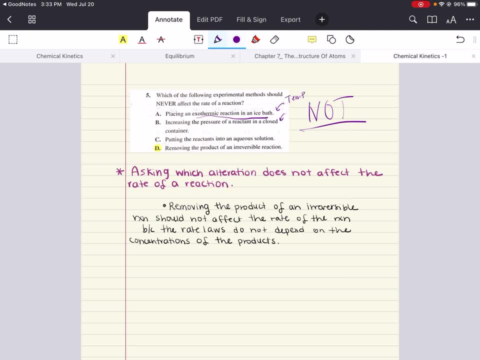 bath. So, essentially, temperature, All right. Increasing the pressure of a closed container, All right. So this is giving us pressure, Putting the reactions into an aqueous solution. So this is changing solvent, if you will, All right. And D says removing the product of an irreversible. 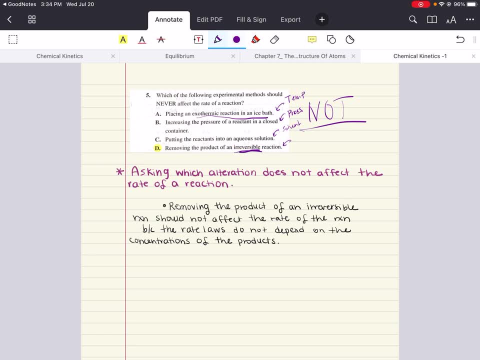 reaction. So this is changing solvent, if you will, All right. And D says removing the product of an irreversible reaction. All right. So off the bat temperature. we talked about this in the first problem. Temperature directly affects the rate constant K. So that automatically makes A not the correct answer. 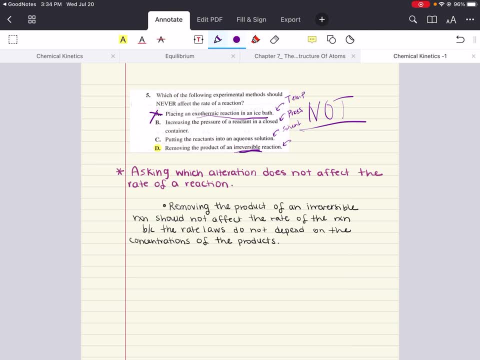 All right. Changing the partial pressure of a gas, like stated in B- all right, will affect the number of effective collisions per time, All right, And that kind of consequently also alters the temperature. So B is not the correct answer, All right, Note that concentration changes, I'm sorry. Note that changing the partial pressure. 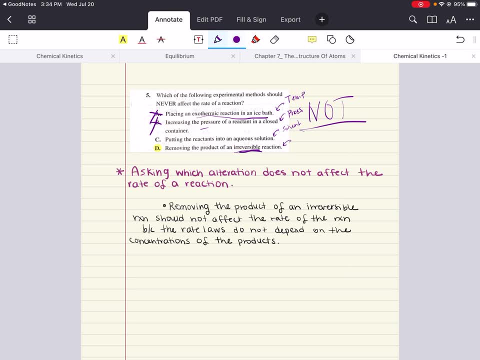 partial pressure. try saying that 10 times fast. Changing the partial pressure of a gas is gonna affect the number of effective collisions per time And that is going to affect the rate of your reaction, how fast it will proceed or how slow. All right, So that's not correct, All right. 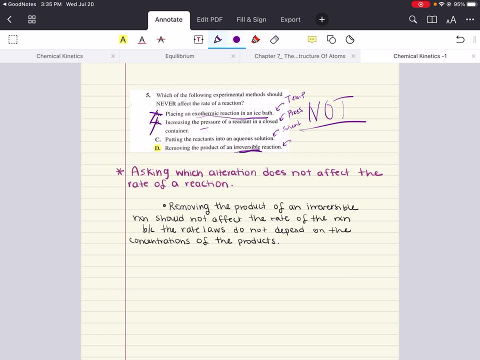 Now solvent Actually also affect the rate of reaction. What you put your reactants in, what kind of solvent- whether it's water or ethanol, blah, blah blah, That's actually also gonna affect the rate of reactions. Okay Why? Because your reactants interact with the solvent- different solvents- 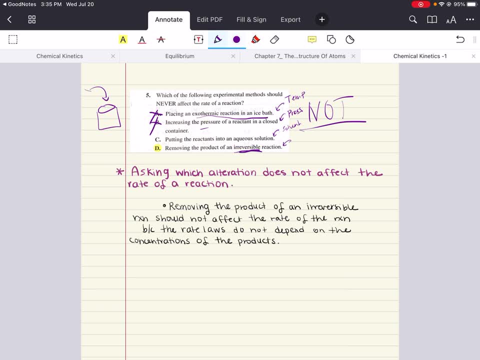 in different ways And that's gonna either speed up or slow down the process. All right, Depending on your solvent. So solvent have an effect on your rate of reaction. All right. So temperature pressure, solvents: these first three answer choices. 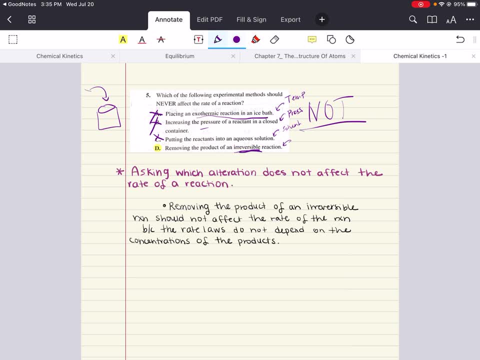 here all have an effect on the rate of reaction. All right Now, removing the product of an irreversible reaction. irreversible which means it only goes from reactants to product. There's no going back and forth to reach equilibrium. All right, Removing the product of an irreversible. 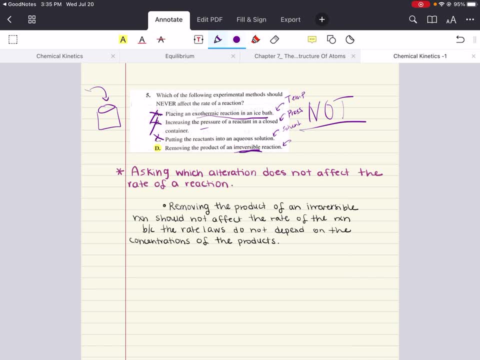 reaction is actually not going to affect the rate of reaction Why? Because the rate law does not depend on the concentration of products. Our rate loss only depend on the of reactants. We've written our rate laws right: Rate equals rate constant times reactants. 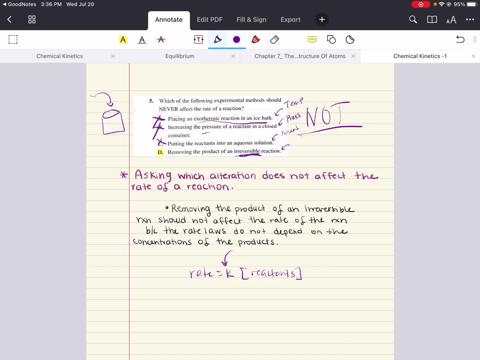 All right. Now we've talked about what affects the rate constant, right? Because obviously the rate constant is in our whole equation. So if you alter the rate constant, you alter the rate equation, You alter the rate of reaction, temperature, pressure, solvent, those all affect. 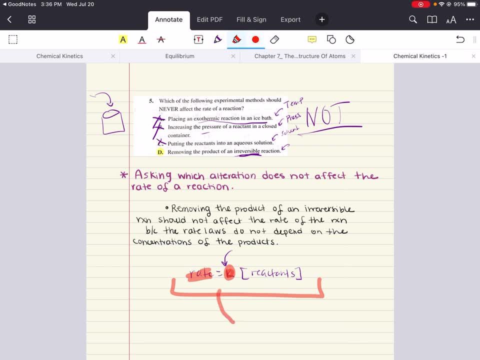 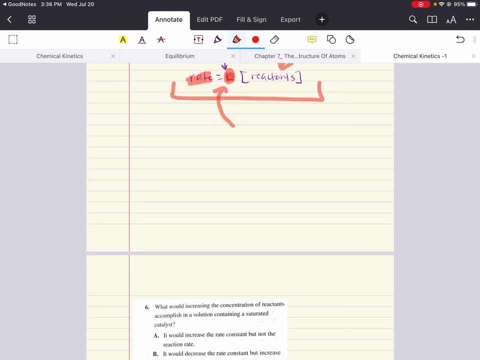 K, All right. But guess what? Products don't affect K and products are not reactants. So removing the product is not going to affect your rate of reaction. Removing product is not going to affect it. Fantastic. So the answer is D, All right. Six says: what would increasing the? 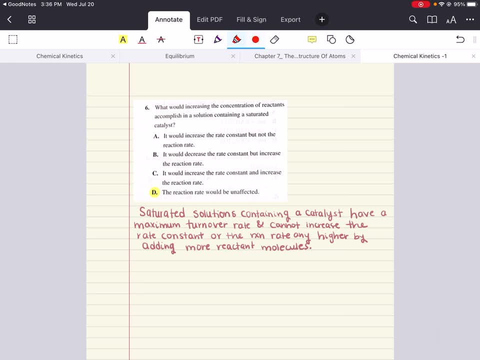 concentration of reactants accomplish in a solution containing a saturated catalyst? What would increasing the concentration of reactants accomplish in a solution containing a saturated catalyst? What would increasing the concentration of reactants accomplish in a solution containing a saturated catalyst? Well, this is interesting. Now we know, while increasing the concentration 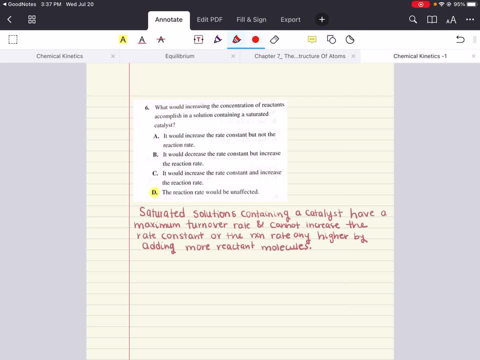 of reactants can alter the reaction rate in, say, first, second or any higher order reactions- saturated solutions that contain a catalyst. they have the maximum turnover rate and they cannot increase the rate constant or the reaction rate any higher by adding more reactant molecules. All right, So I have that. 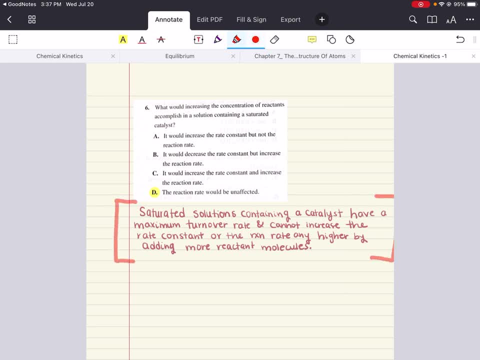 written here because this is an important note to keep in mind. All right Saturated solutions containing a catalyst are going to have a maximum turnover rate, So we're not going to be able to increase the rate constant or the reaction rate by adding more reactant molecules. That makes sense. 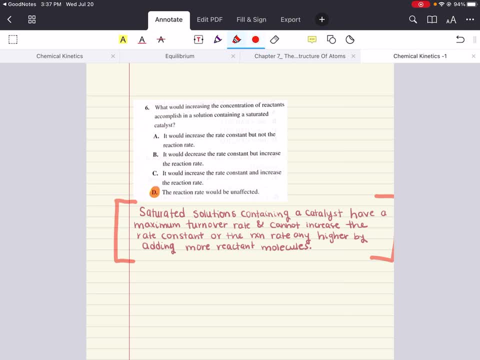 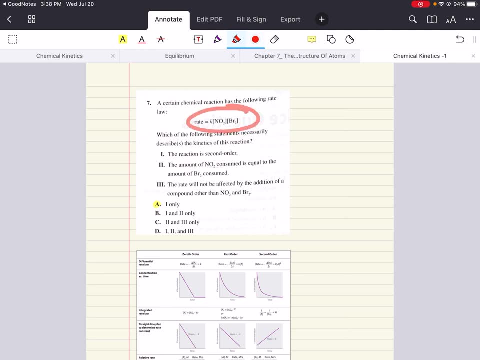 That makes the answer choice for six: D. Fantastic Seven says a certain chemical reaction has the following rate law: All right, Awesome. Which of the following statement necessarily describes the kinetics of this reaction? Let's read these answer choices. All right, Let's go one by one: The: 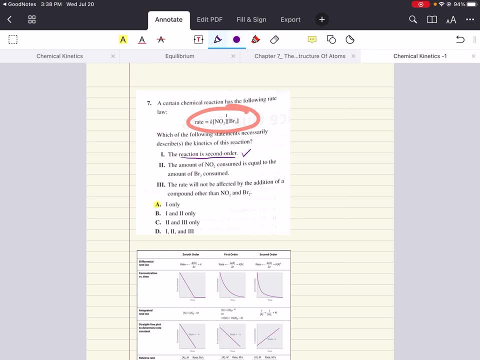 reaction is second order. Guess what? That's correct. We have a one exponent here on NO2 and one on Br2.. Usually one is not exponent, So we have a one exponent here on NO2 and one on Br2.. If it's not explicitly written, we know that it has to be one. All right, What's one plus one? 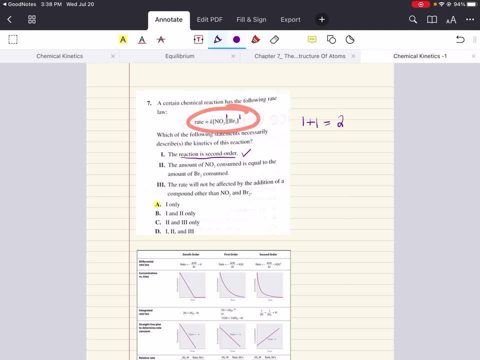 Two, Our reaction is second order. That's correct. Two says the amount of NO2 consumed is equal to the amount of Br2 consumed. All right, That's interesting because the exponents in the rate laws are unrelated to the stoichiometry coefficient. 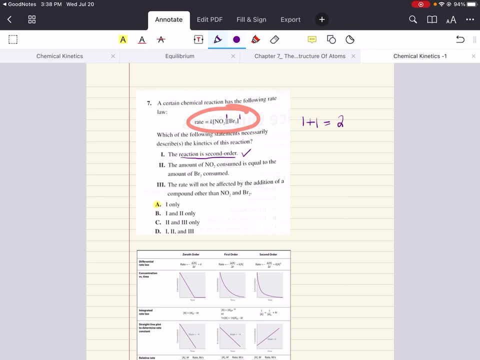 So NO2 and Br2 could have any stoichiometric coefficients in the original reaction and still be second order, And so you really actually can't say that this is true unless you had the whole reaction and more information. So that is incorrect. Now statement three says: 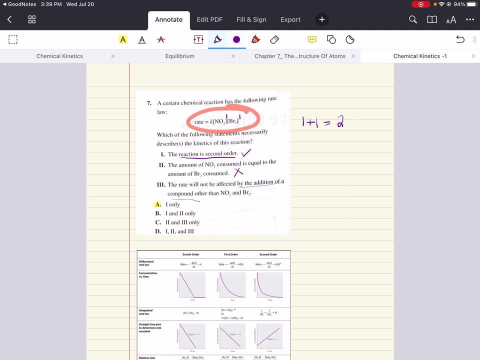 the rate will not be affected by the addition of a compound other than NO2 and Br2.. So that's incorrect, because- guess what? The rate can be affected by a wide variety of compounds. The best example: A freaking catalyst, All right. So that's also not true. The only true statement is one, And 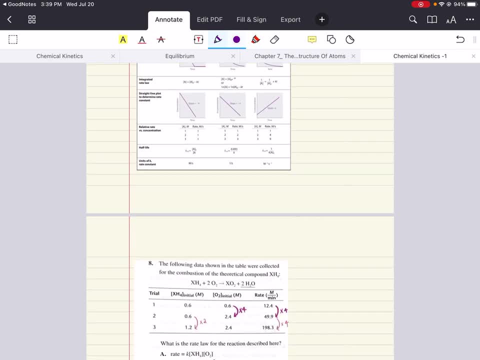 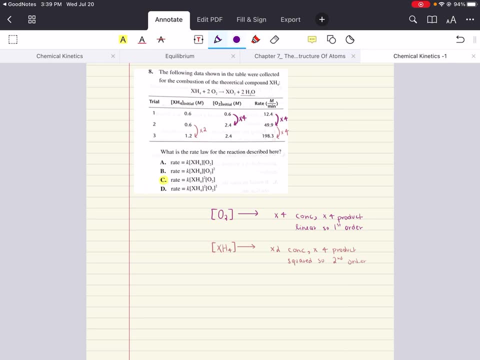 so A is the correct answer. Fantastic, Let's do eight. The following data, excuse me. the following data shown in the table were collected for the combustion of the theoretical compound X- H4.. What is the rate law for the reaction described here? Fantastic, Well, we have our. 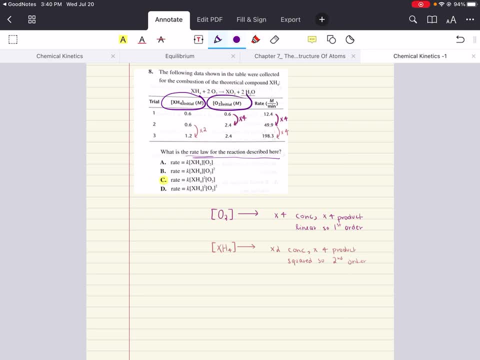 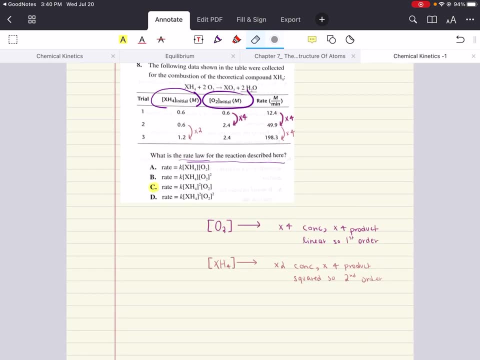 two reactants Here, they are Okay And we're shown. we're shown something interesting here. All right, How changing concentrations? all right, of each in different trials, how they affect the rate. Okay, So first of all we start off with 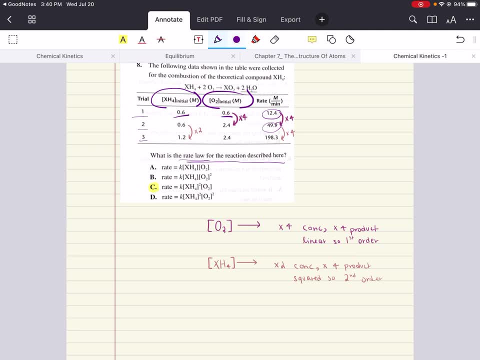 what is the rate of X- H4, equal molar concentrations of both 0.6 molar X H4, 0.602.. Perfect, And the rate is 12.4.. Cool, This is a good starting place. That's their first trial Important. 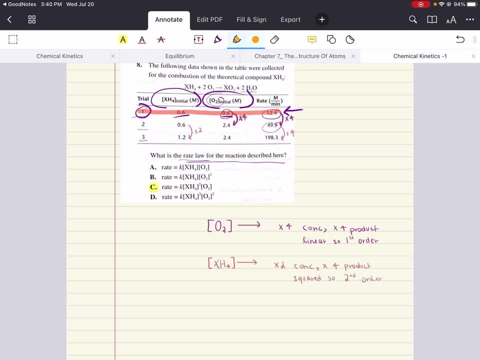 information for us to keep in mind. All right, What about their second trial? In their second trial, what do you notice? They keep the same concentration of X H4 as the first trial, but they change the concentration of X H4 as the second trial. So what do you notice? They change. 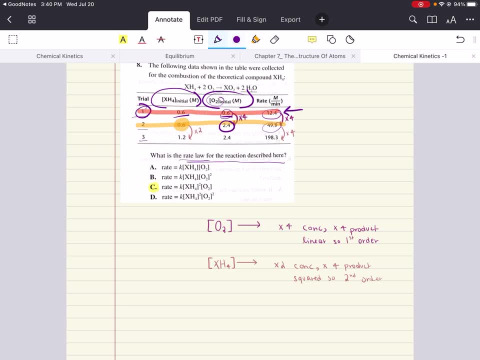 the concentration of X H4 as the first trial. but they change the concentration of X H4 as the first trial, but they change the concentration of O2 in the second trial. By how much? Four times, four times as much. All right. So we go from 0.6 concentration of O2 to 2.402.. And that's the only. 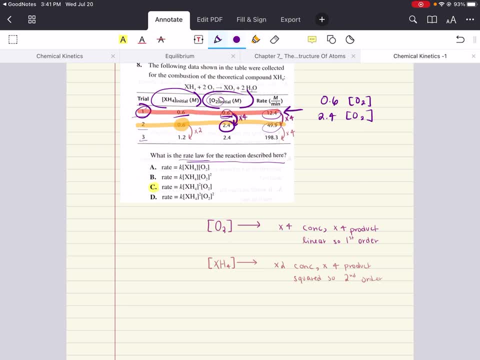 thing they changed between trial one and trial two, Cool. So what we notice is they've multiplied the concentration by four. What happens to the rate when they do that? The rate also increases by an order of four. All right, So the rate from trial one to the rate for trial two, when only changing the. 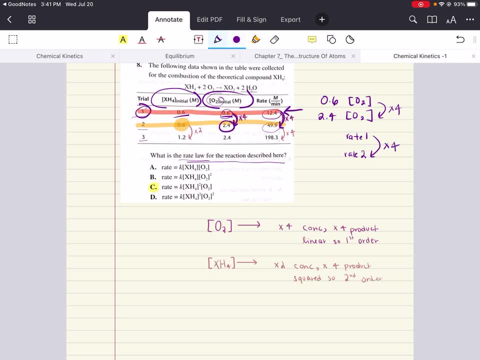 concentration of one reactant changes by an order of four? What do we call a reaction where, when you change the concentration by a factor, the rate changes by the same factor? That's a first order reaction, All right. So O2, right off the bat- now we know, all right- has a coefficient of one. 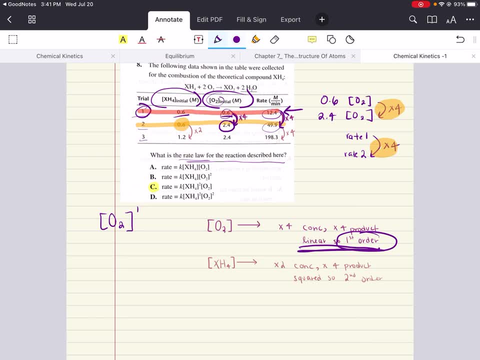 All right, order. o2 is first order. cool, fantastic. let's look at their third trial. all right, in their third trial, what do we notice? well, what we notice is they keep the same concentration for o2 as their second trial. all right, so trial two and three: the o2 has the same concentration. good, all right. but 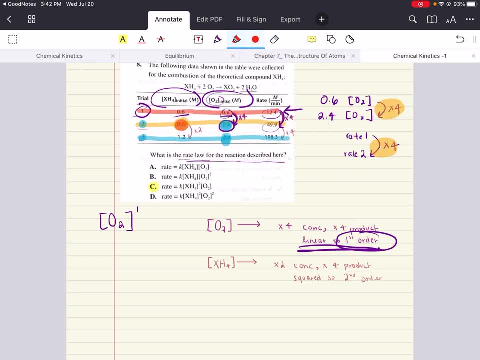 they change the concentration of xh4. they go from 0.6 to 1.2. all right, so they go from 0.6 to 1.2 for x, for xh4, all right, cool, that's the concentration. what happens to the rate? 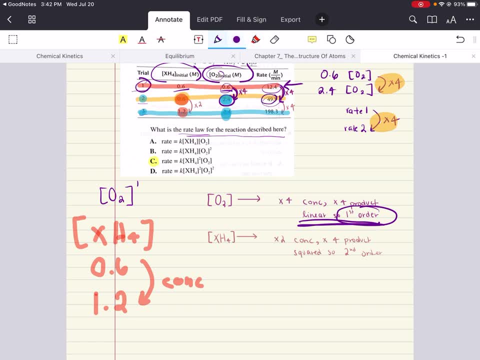 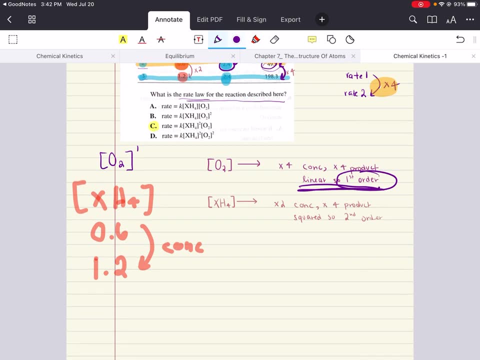 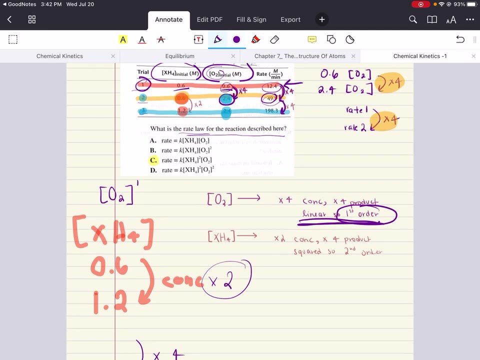 all right. well, the rate changes from 49.9 to 198.3. all right. the concentration changes by an order of four. so here the constant. so here what's happening is we're doubling the concentration of xh4 times two and the constant and the rate. 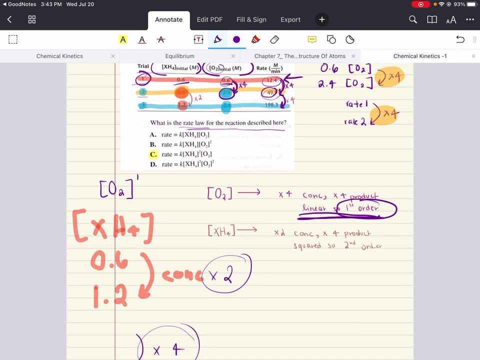 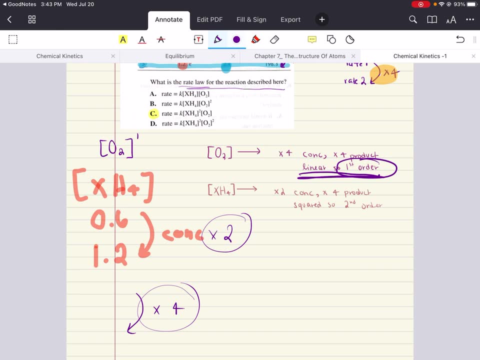 is changing by four. all right. so what kind of reaction changes? uh, changes the rate in a squared manner, all right. when you double, say, for example, if you multiply by two the concentration, the rate changes by two squared. oh, that's a second order reaction. all right, so o2 is a first order. 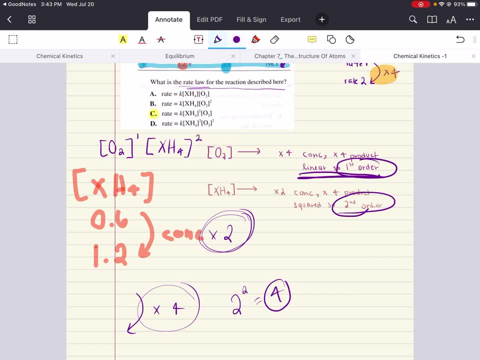 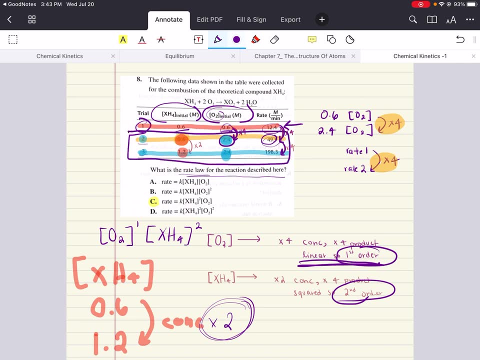 reaction xh4 is a second order reaction. now, the reason why all right, the reason why we were using two and three for xh4 is because all right, is because we want similar concentrations, for one thing, at least when we're comparing two reactions to figure out the order of a reaction. 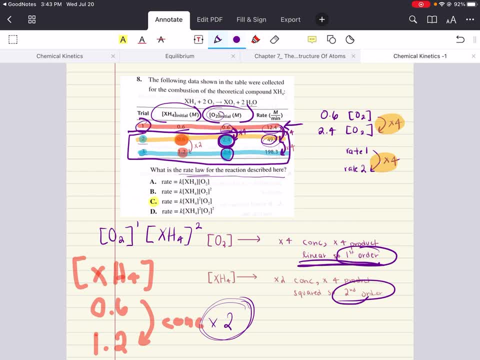 all right. so that's why in the first two trials- we took those- the concentration of xh4 is held constant, all right, only the concentration of o2 is changed, perfect. so then we can compare. when we compare the rates of the first and second trial, we know that the only effect on that rate can be. 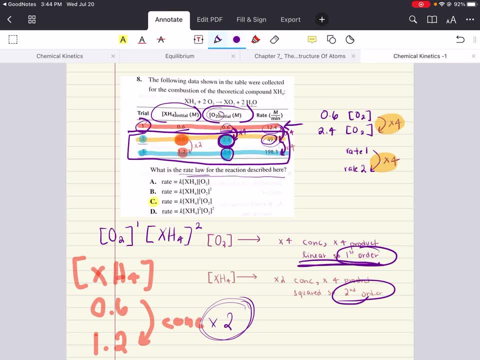 because of o2, because only the concentration of o2 is changed. then we looked at trials two and three for xh4. why? well, because uh, o2 concentration is held constant. so then we can say that the rate changes from two to three simply because we change the concentration of xh4. and those two things are. 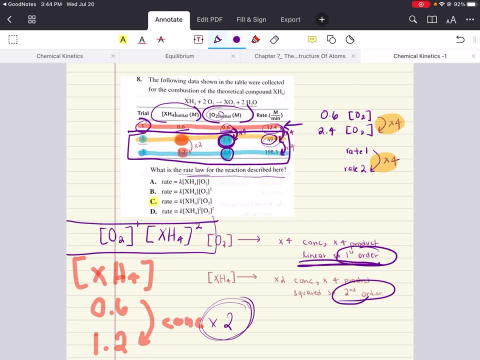 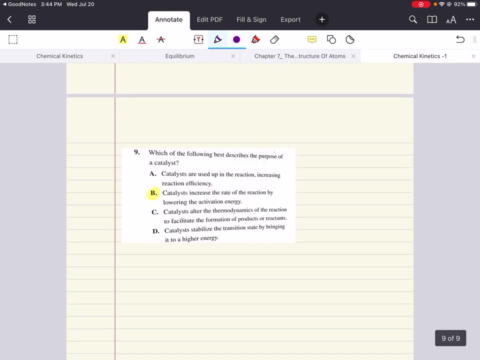 going to help us realize the true order of each reactant and the total rate equation for this reaction. the answer is c, fantastic. let's move on to our last and final question, a nice concept question to end this. all. which of the following best describes the purpose of a catalyst? 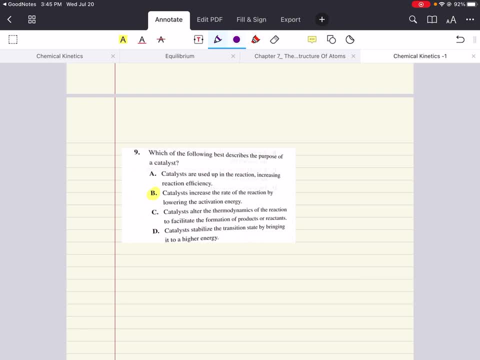 by definition, a catalyst increases the rate of a reaction by lowering the activation energy, making it easier for both the forward and reverse reaction to overcome the energy barrier. all right, catalysts are not used up in a reaction. they do not alter the equilibrium of a reaction, all right. so those are important things to keep in mind because they help you.